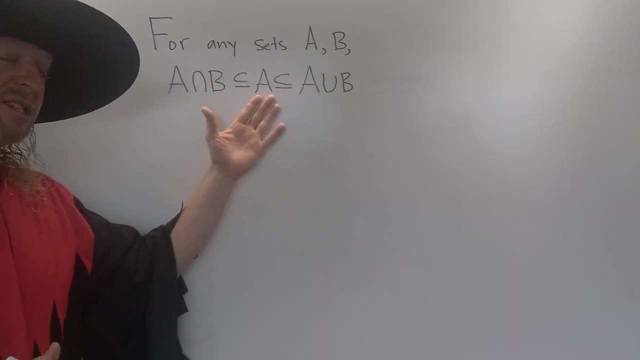 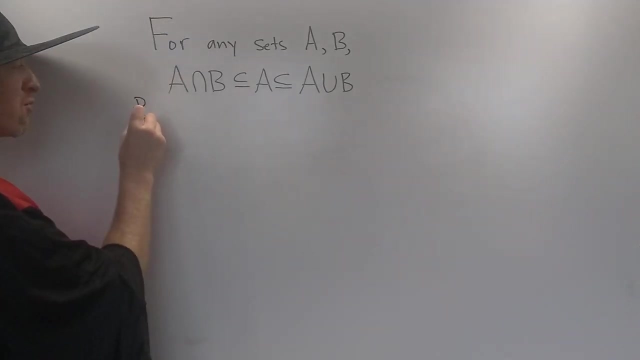 Hey, what's up In this problem? we're going to prove that A intersection B is contained in A, which is also contained in A union B. okay, Let's go ahead and go to the proof, So, proof. So we'll start the proof by showing the first inclusion. We'll show that A intersection B. 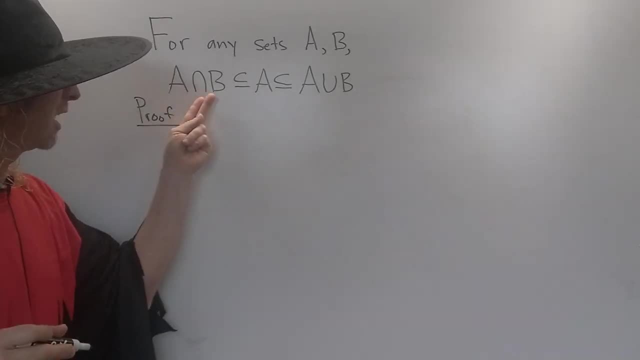 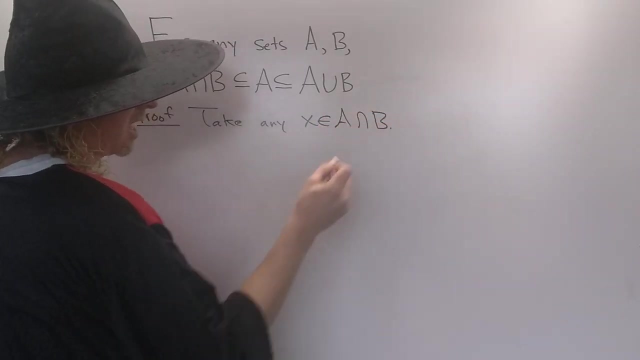 is contained in A. okay. So to do that, we'll take an element in A intersection B and we'll show it's also in A. So if we can show every element here is also here, we're done. So take any x in the intersection, So any x in A intersection B, And now we have to show. 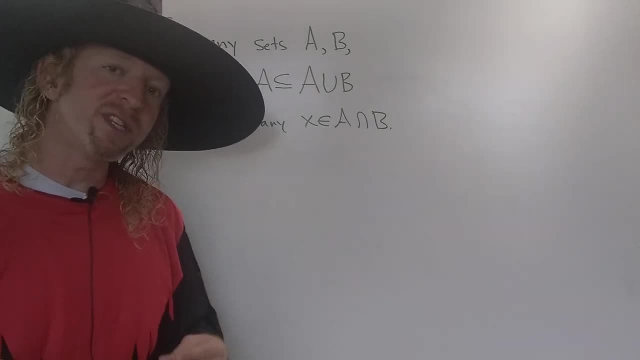 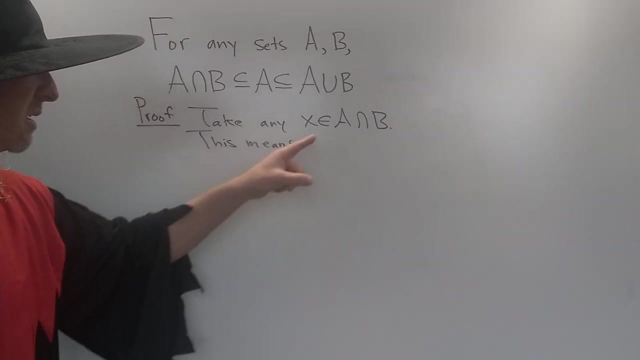 that it's also in A. So now we use the definition of intersection, right. So this means so. this means so. what does it mean for x to be in the intersection? Well, it means it's in A and it's also in B. So this means x is in A and x is in B. 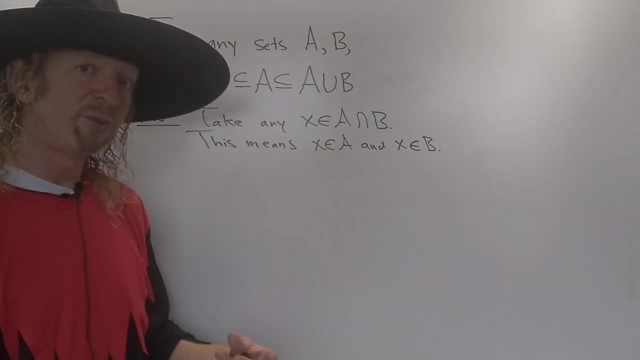 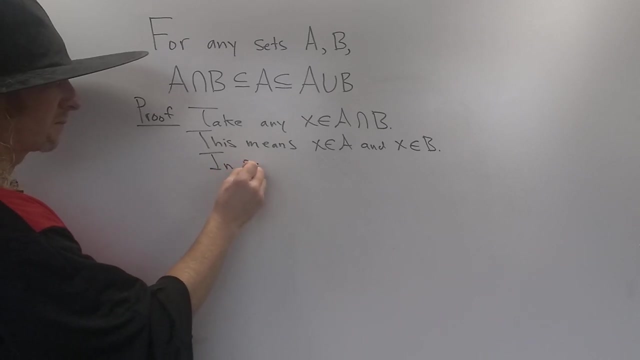 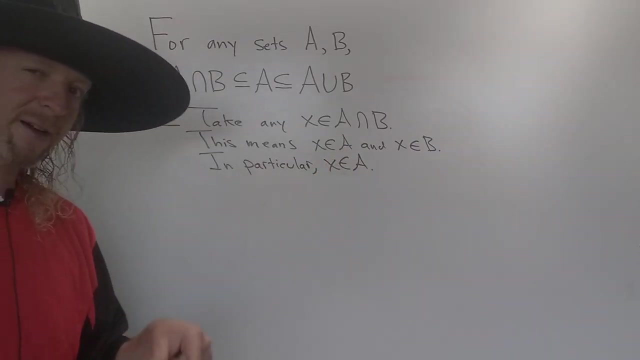 So we want to show it's in A, So it's already written here. So what we can do is we can emphasize that by using a specific language. We can say something like, in particular, x is in A right Isolate, but that's the fact that we want to emphasize, So we took an x in. 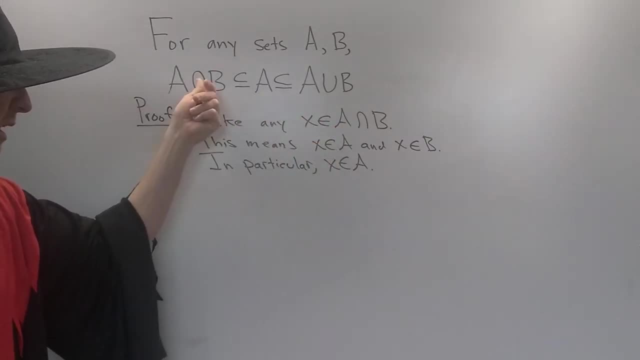 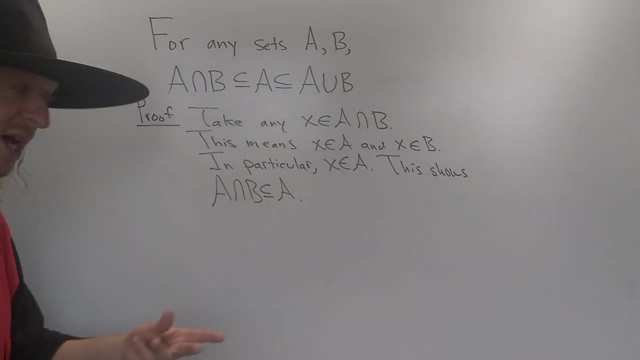 intersection, We show it's in A. Therefore the intersection is contained in A, So this shows. this shows that A- intersection B- is contained in A. Now we have to show that A is contained in the union, So we'll do it again. 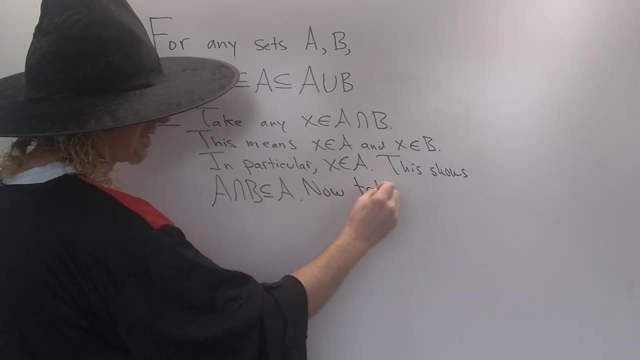 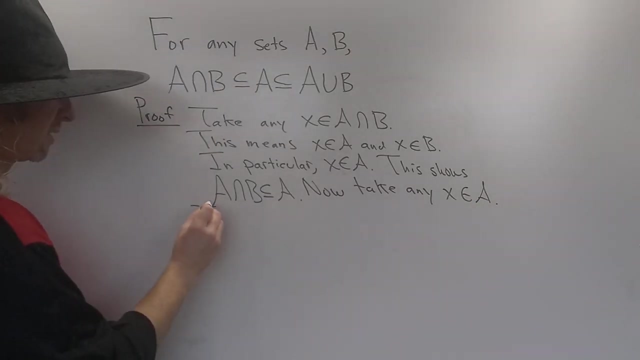 So now take any x. We could have used the same x, but let's start over. So now take any x in A, And now we have to show it's in the union. So here's the trick. This means: 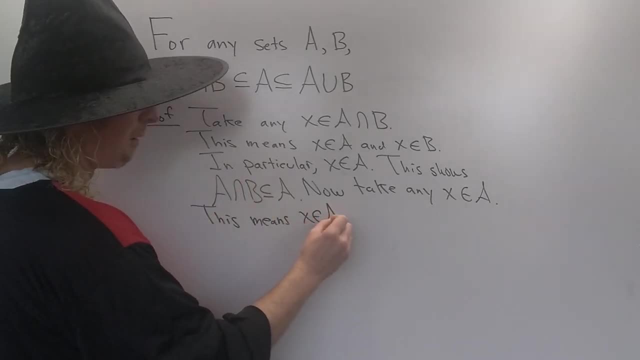 this might not make sense, but I'll explain it. This means x is in A or x is in B, So you may say what? How do you know it's in B? Ha, I didn't say that, right. 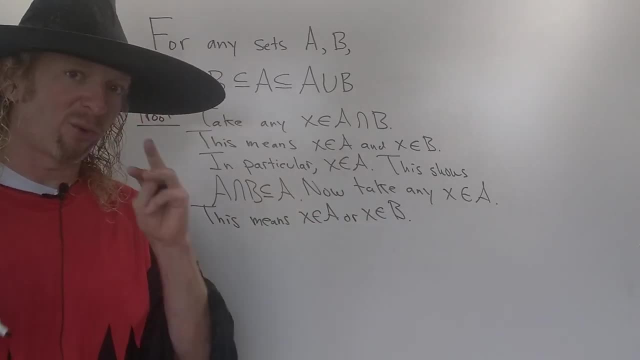 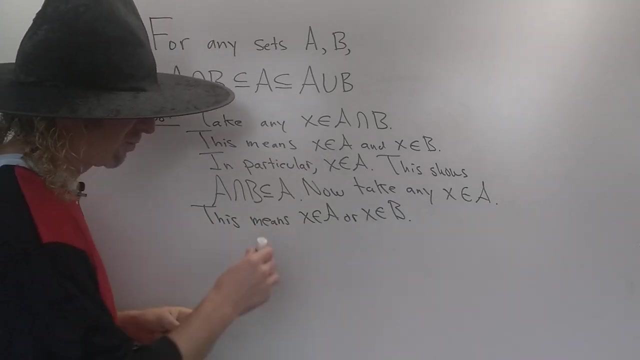 So an or statement in mathematics is true under one of the three conditions: Either x is in A, it's in B or it's in both. So or is inclusive and it's true under three conditions. Either this is true, this is true, or they're both true. Well, x is in A, So the first condition is true.